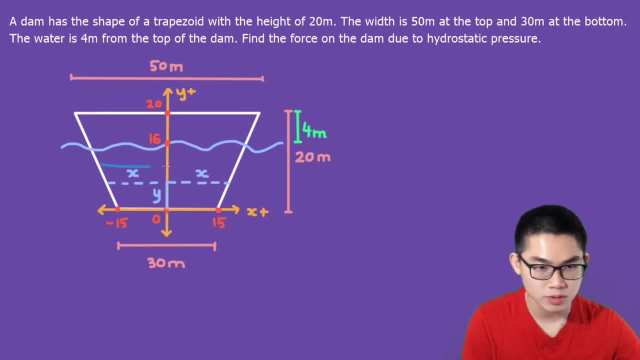 stripe, then this stripe. so you get the idea. we keep doing that until we reach the surface of the water and then we add all of those forces together which gives us our hydrostatic force. so let's say that this is our stripe. let's say this is our stripe, then the distance from the 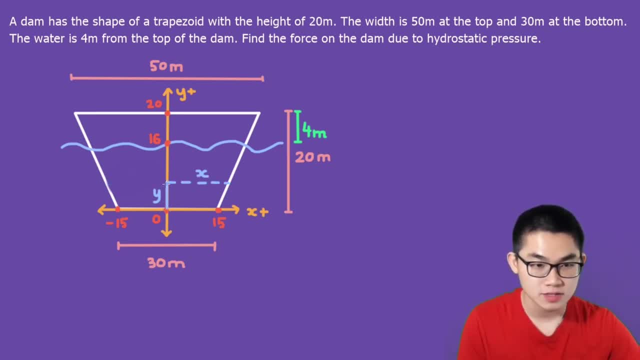 center to our stripe is y. the distance from here to here is going to be x. but we also know that because the y-axis divides this shape in half, then the distance over here is also x. the distance from here to here is going to be x. the distance from here to here is going to be x. 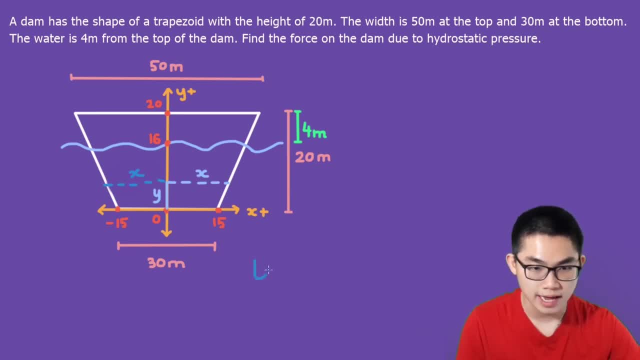 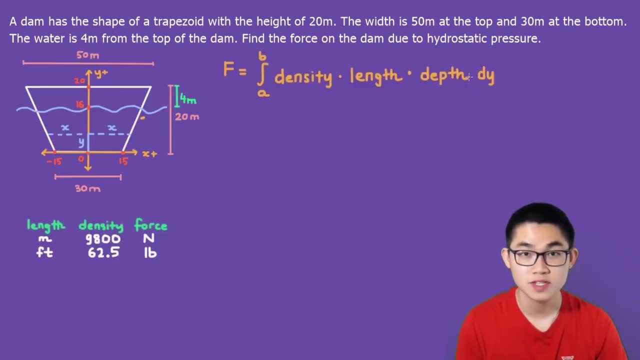 so the total distance of the stripe, or the length, is equal to 2 times x. and here is the formula to calculate the hydrostatic force. and let's solve this formula together. so what is a and what is b? well, we want to find the hydrostatic force act because of the 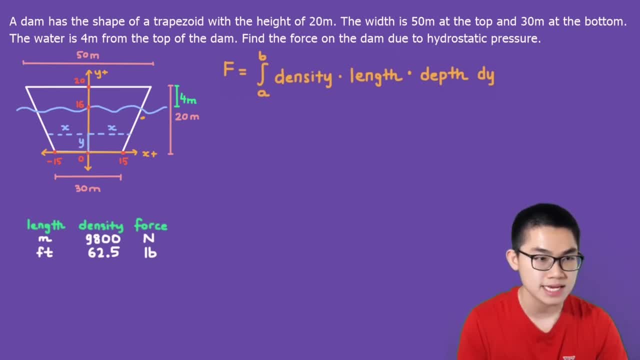 water, which is from here to 16. right, so a is 0 and b is 16. what is the density? well, i've put this table here and because the problem is in meters, then the density will be 9800. the density will be 9800. 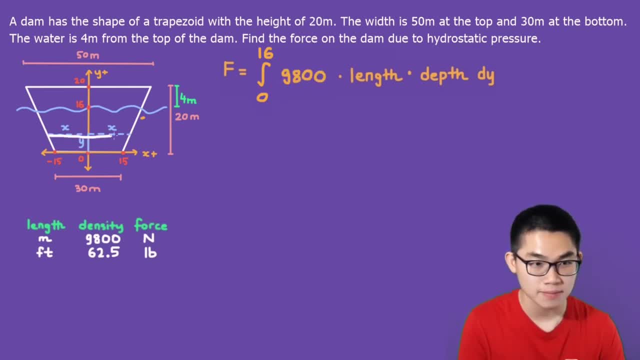 how about the length? well, we want to find the length of the stripe and, as mentioned before, it's going to be 2x, but the formula wants everything to be in terms of y, so we have to convert the x to the y, and let me show you how to do it. if you look here, this point: 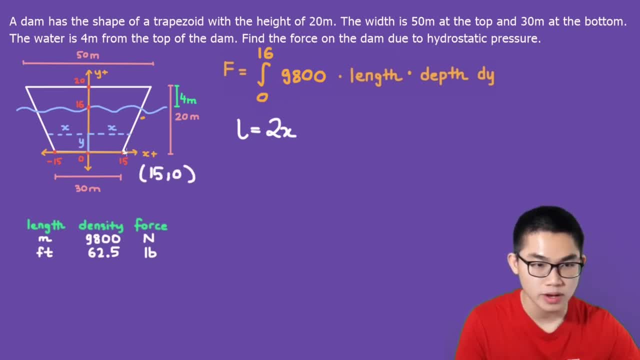 is going to be 15: 0, right? this is the point on the x and the y axis. so let's write it out. how about this point here? well, the distance from here to here is half of 50. we know that from here here is 50, so from here here is 25 and the height is 20.. 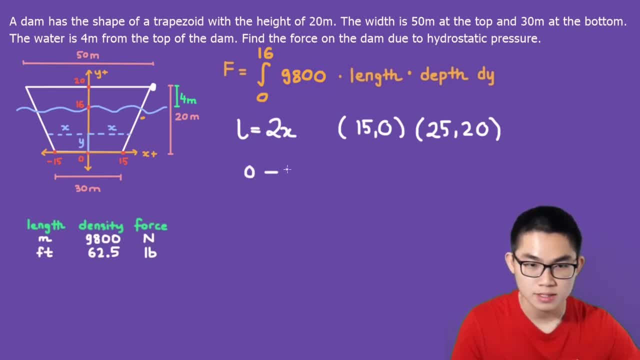 let's calculate the slope. we get 0 minus 20 over 15 minus 25, that's going to give us negative 20 over negative 10, which is going to be 2, and using the linear formula, we have the slope 2x plus b and we have to substitute one or these two points. let's substitute this one, so the y 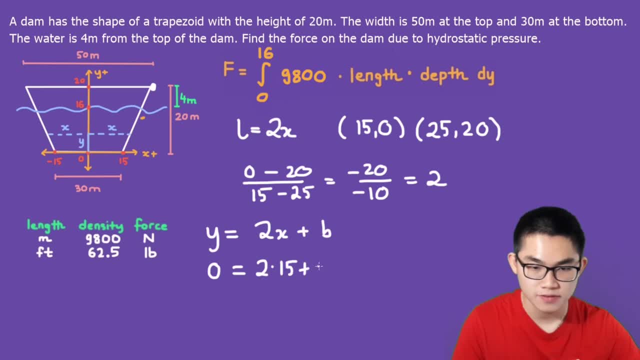 is 0, x is 15. so 2 times 15 plus b, b is going to be negative 30. so we get: y is equal to 2x minus 30.. let's solve for x. so in this equation that we just found out, we get: y plus 30 is equal to 2x. 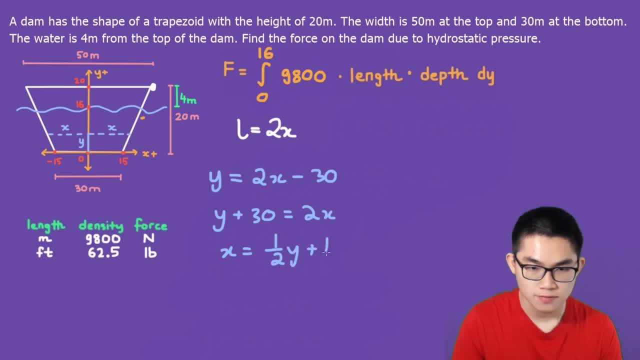 and then x is going to be 1 over 2y plus 15.. so the length is 2x, which means 2 times 1 over 2y plus 15. that's going to be y plus 30.. let's put it back into the length here. last but not least, we need to find the depth. 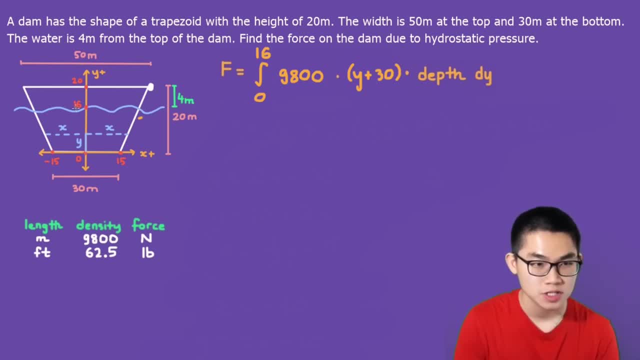 so the depth is the distance between our stripe to the surface level of the water. so that's going to be this distance. we want to find this depth right there. well, first things first, we know that the distance let's use- let's use yellow this time- so the 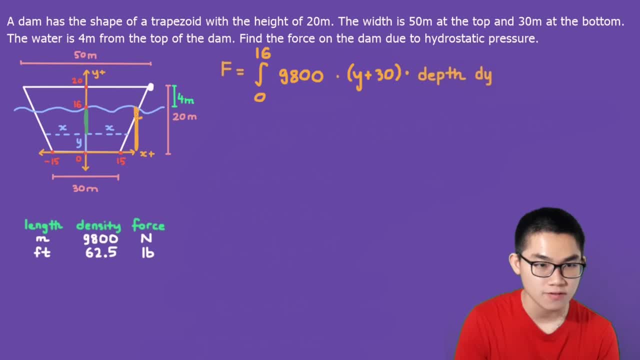 distance between the x-axis to the surface level of the water. that's going to be 16. right, you can see here: 0, that's 16. so the yellow distance is going to be 16.. well, if we take the yellow distance and we minus y, we're going to get the green distance. so the depth is just basically. 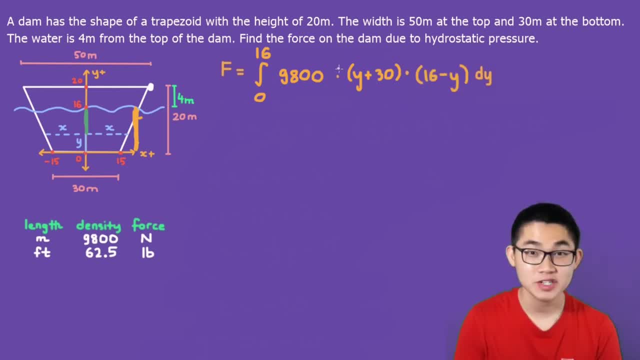 16 minus y. this integral is very easy to do, so let me save you your time and after you solve it, you should get 4.4 times 10 to the power of 7.. and what's the unit? well, looking at this table, the problem is in meters. so the final answer is the force, which is newtons. in the next, 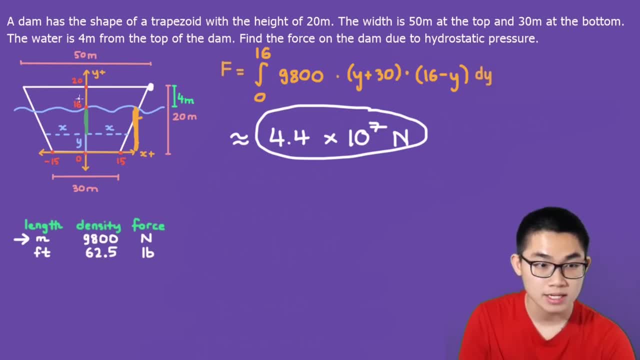 video i will show you how to calculate the hydrostatic force when the shape is a circle. we've got orange, which means it's a circle, and blue, which makes it 4.7 meters for the 2nd time. so i'm just gonna use this target and i'm telling you that it's actually a circle.